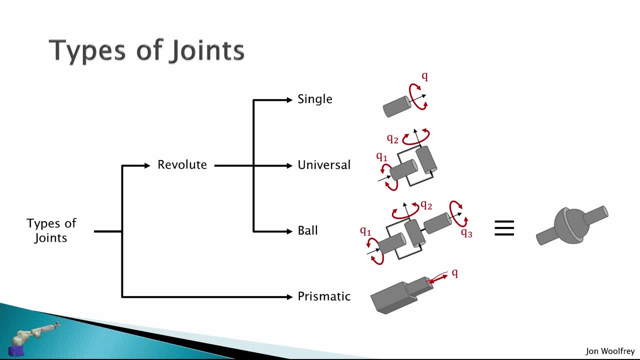 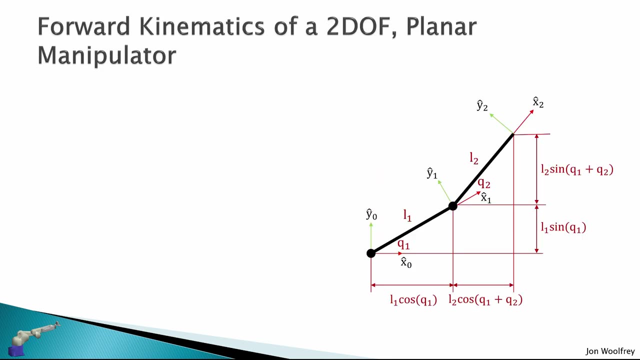 So these translate along this axis of actuation here. So when we develop a robotic kinematic structure, we have different combinations of these types of joints in sequence. So let's look at the forward kinematics of a 2DOF planar manipulator as given in this diagram here. 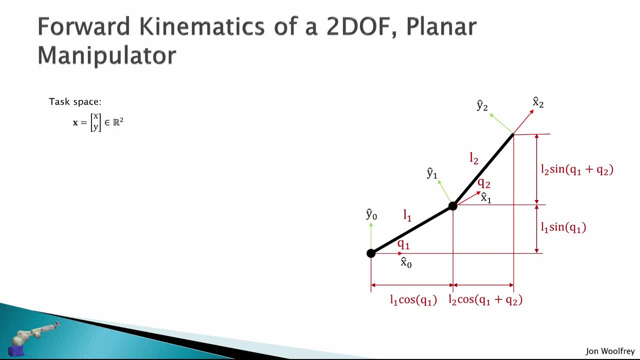 So the task space we say is given by the X and Y position of the end effector And we say that it is in the set of real values in two dimensions And the joint or control space of the robot is Q, which is given by Q1, Q2 in the set of real values in two dimensions. 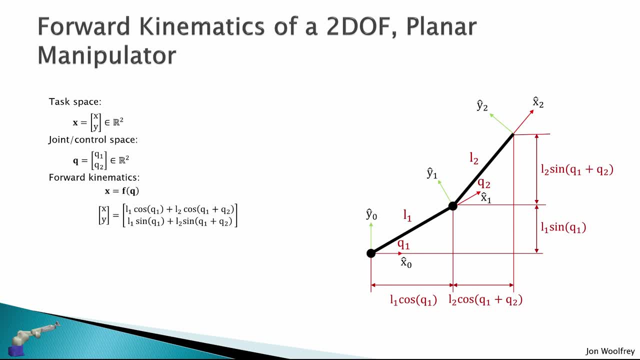 Then the forward kinematics is: X is a vector function of Q will be L1 cos Q1 plus L2 cos Q1 plus Q2.. So this is X, And then Y will be L1 sin Q1 plus L2 sin Q1 plus Q2.. 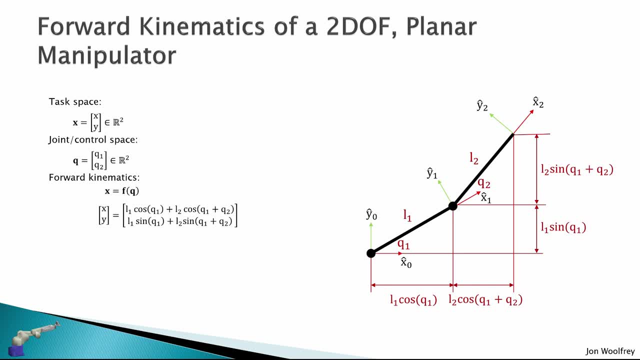 So this is Y, And then Y equal to X, Simples. But what about orientation? Well, we can just combine Q1 plus Q2 will give the orientation Phi oh, Psi, sorry here, And we just append the task space with Psi at the bottom. 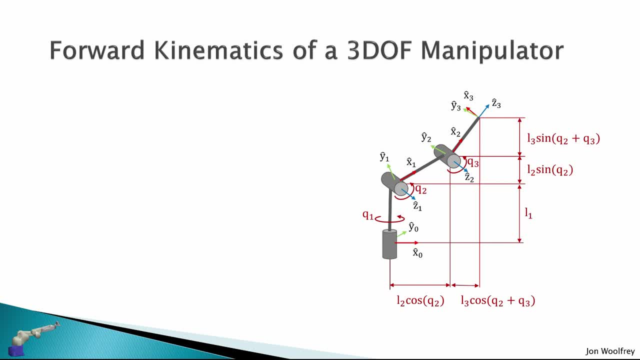 Let's take a look at a more complex example. So we have the forward kinematics of a 3DOF manipulator. So the task space is given by x, y, z in the set of real dimensions and the joint control space is q1, q2 and q3. 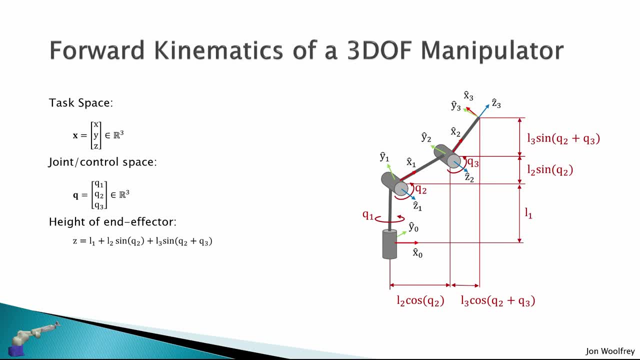 So the height of the end effector will be the z direction, which is L1 plus L2 sine q2 plus L3 sine q2 plus q3. here And then we also need to consider the distance of the end effector projected on the x y plane. 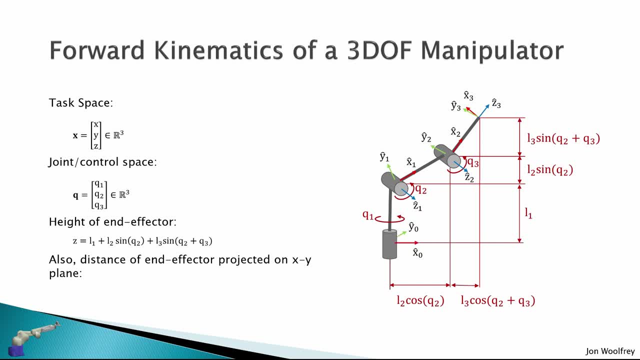 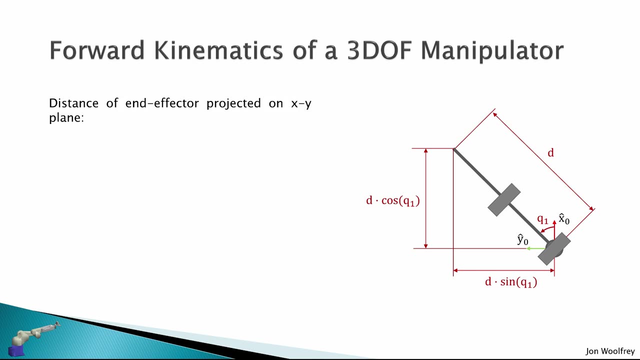 So we're projecting on this plane here and this is given by L2 cos q2 plus L3 cos q2 plus q3.. So now the distance of the end effector projected on the x y plane, as we previously defined as d, was L2 cos q2 plus L3 cos q2 plus q3. 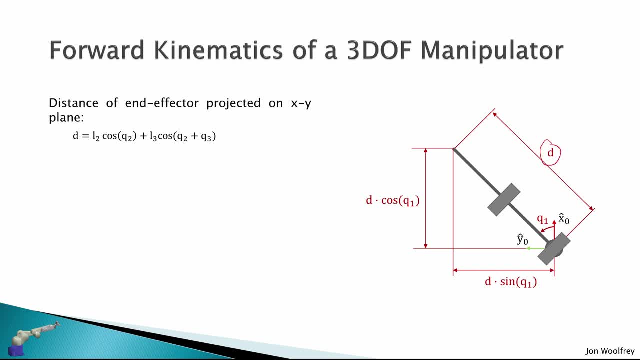 So here we're looking at the robot from the top view and that's the distance d, and so the x and y position of the end effector is then d cos q1. here for x, and this is L2 cos q1, cos q2 plus L3, cos q1, cos q2 plus q3.. 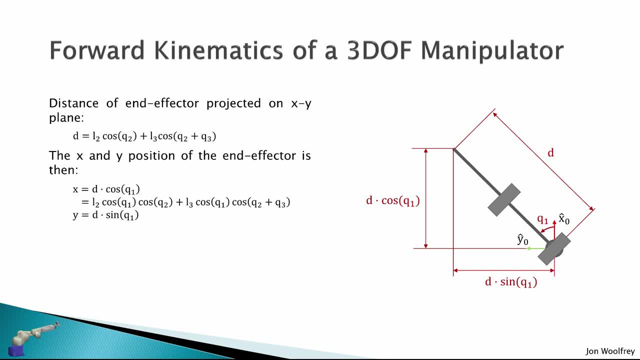 And similarly y is equal to d sine q1.. And it is given by this solution here. So we just multiply again d by sine q1.. And therefore the forward kinematics as a vector function of q is x, L2 cos q1, cos q2 plus L3, cos q1, cos q2 plus q3.. 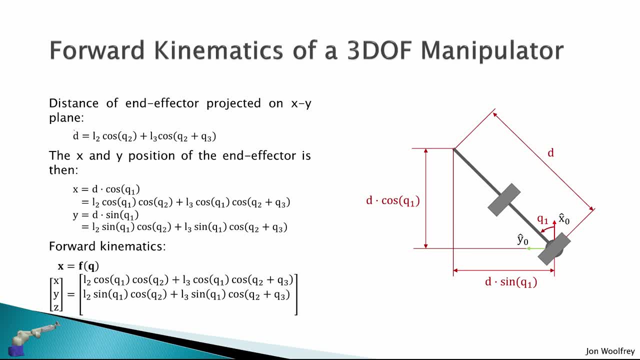 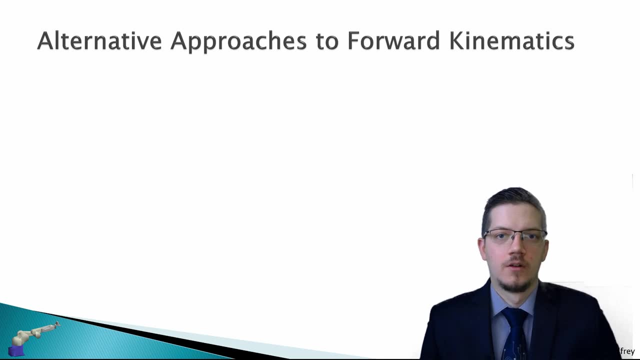 y is L2 sine q1 cos q2 plus L3 sine q1 cos q2.. And z is L1 plus L2 sine q2 plus L3 sine q2 plus q3.. So this is getting much more complicated, Right? so we saw that the 2D planar robot was really simple. forward kinematics. 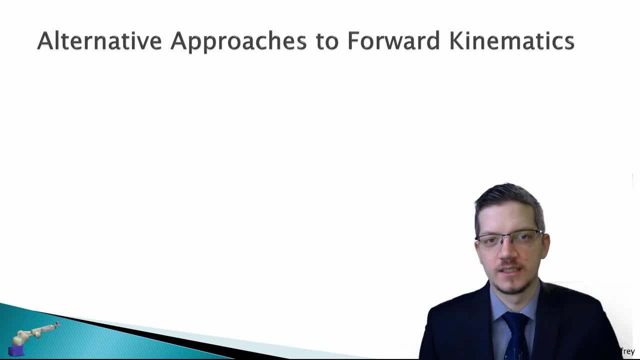 But once we expanded to a 3DOF robot in three dimensions, it started to get very tricky. So the problem is that forward kinematics can be very difficult for complex robot structures, And what we want to do is find a simpler way to derive the forward kinematics. 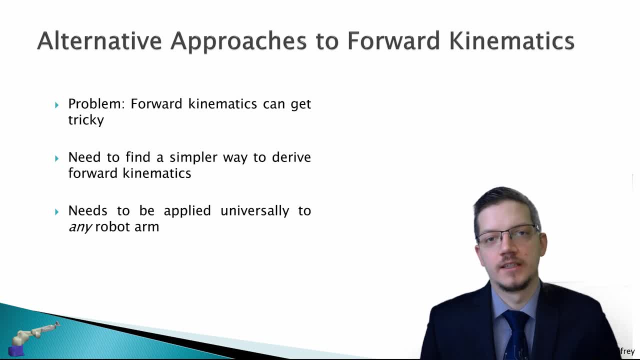 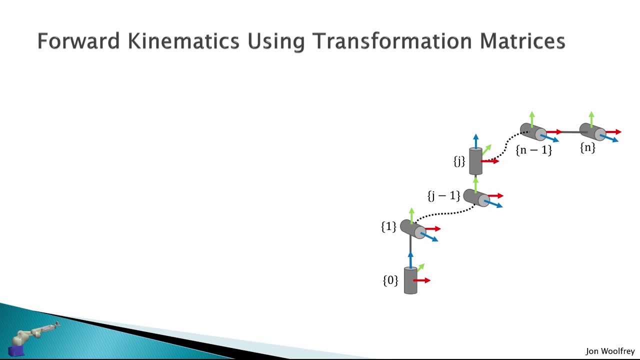 And on top of this it needs to be applied universally to any sort of serial link manipulator. So the power of transformation matrices is that we can derive forward kinematics using them. So we can concatenate transformation matrices between joint frames to determine the end-effector pose. 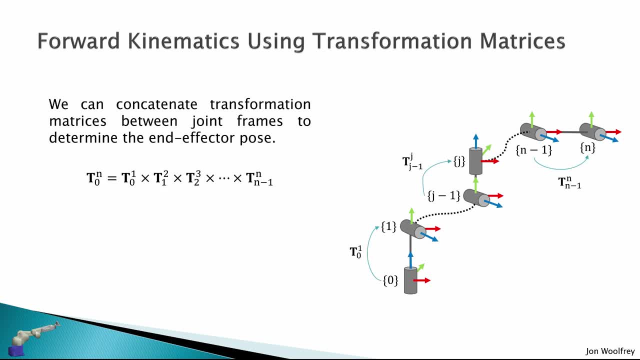 So we just multiply transforms between joint frames all the way up the kinematic structure to get the transform from frame 0, or the base frame to the end-effector frame, Right? so this is just the product: all transforms from j minus 1 to j. 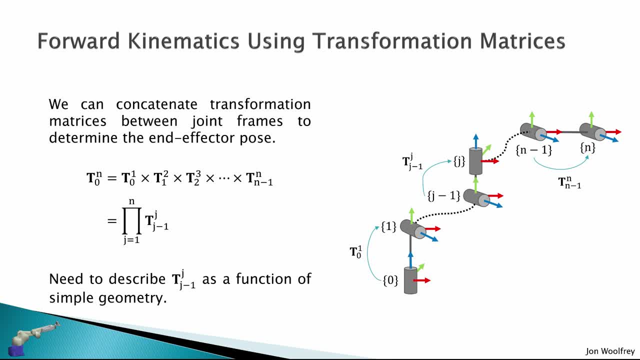 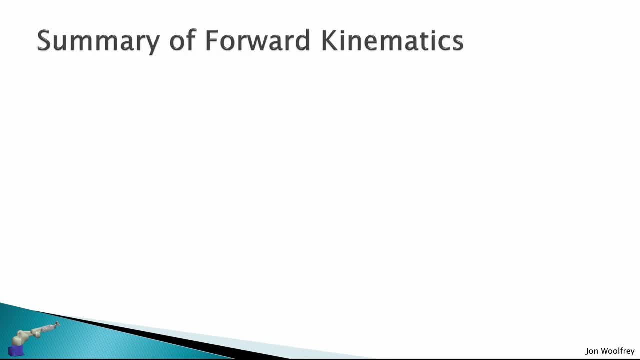 But now we just need to describe the transform from j minus 1 to j as a function of simple geometry. So to summarize this, let's summarize this lecture on forward kinematics. The general forward kinematics problem expresses the end-effector pose x.